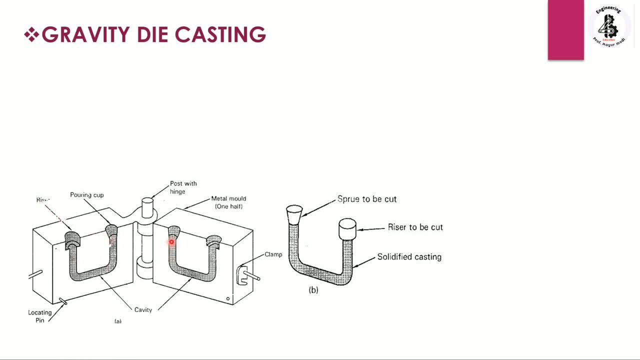 will be our visor and this one is our pouring cup, So basically the molten form of the metals that will be pouring into these ones. So just you can see into the third figure, this is the arrangement of the permanent mold, So by the clampings and all the arrangement. So basically these both the half of the metallic materials. 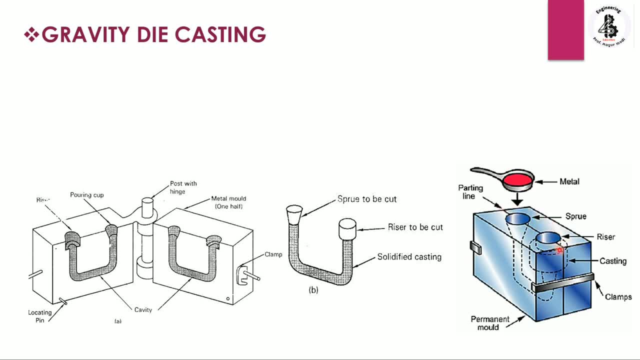 it will be divided by these parting lines. Along with these parting lines, it will be our cast products. So this is nothing, but it will be your permanent mold. So this kind of shape it will be generating with the help of two halves. So this is our molten form of the metals, with the help of bladder that will be pouring into the sprue, So passing through the sprue. 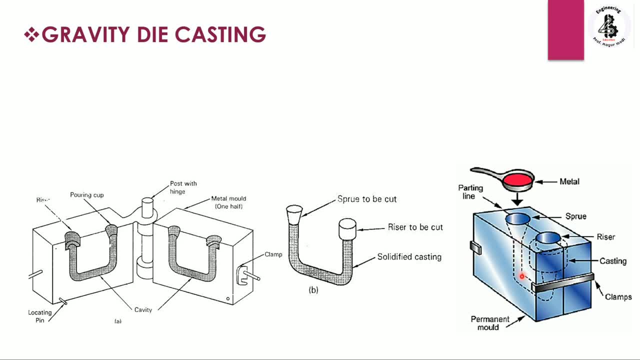 prove that will be entering and with the help of gravitational it will be, fill the cavity and towards a riser. So these risers it will be, gives the 100% ensurement regarding to the 100% filling of the mold cavity. So by the gravity that will be used to making a components, or you can say this is also a 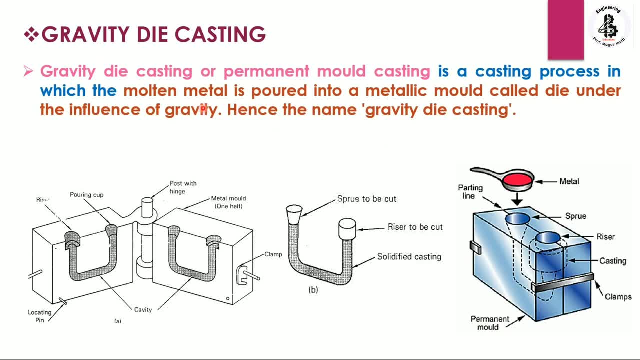 permanent mold casting process. As you can see, the gravity die castings, or permanent mold castings, is a casting process in which the molten metal is poured into a metallic mold called as a die, under the influences of the gravity. So gravity plays a vital role. that's why the name gravity die casting process. 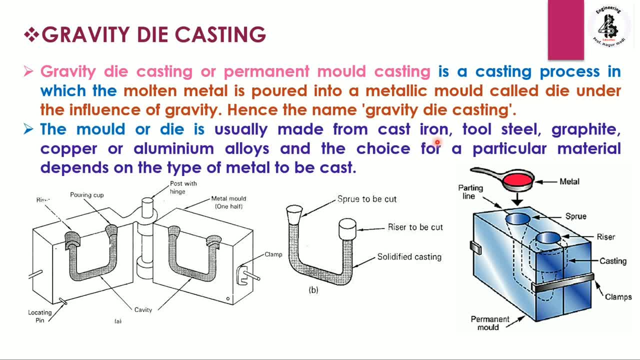 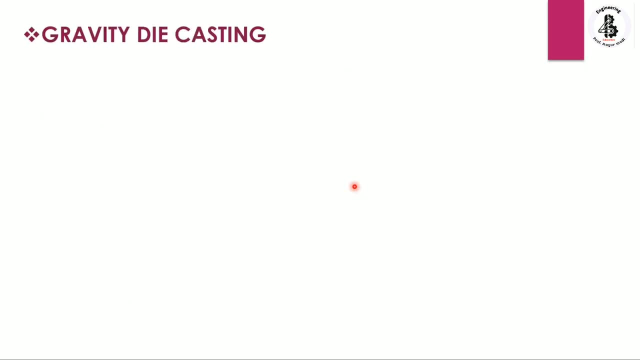 The mold, or you can say die, is usually made from cast iron materials, Toll steels, graphite, copper or aluminum alloys, and the choice for the particular materials depends upon the type of the metal to be cast. Then after, in case of the die castings, just you can see, this is the basic setups. 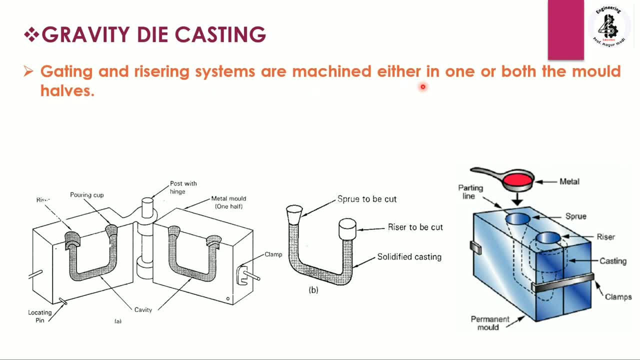 The gating and risering systems are machines, either in one or both the MOHABs that will be depends upon the complexity of the shape and as well as size of that particular mold With particular components. The figure shows a permanent mold made with two halves, which already discussed with resembles. 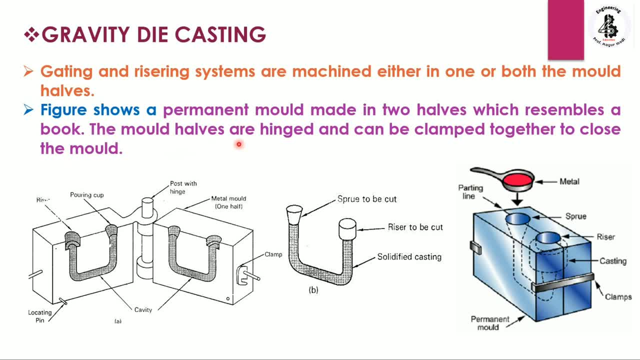 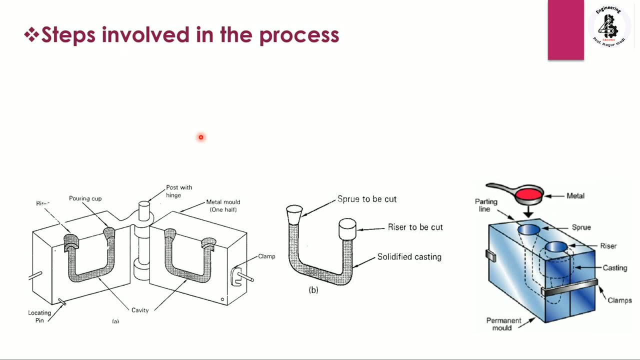 books look like The mold halves are hinged and can be clamped together to close the mold. This is the arrangement we already discussing on to that. So some of the steps is being involving in this process. So this is the setups, So the mold. 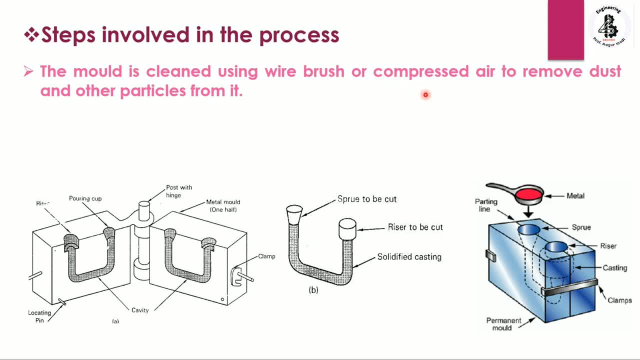 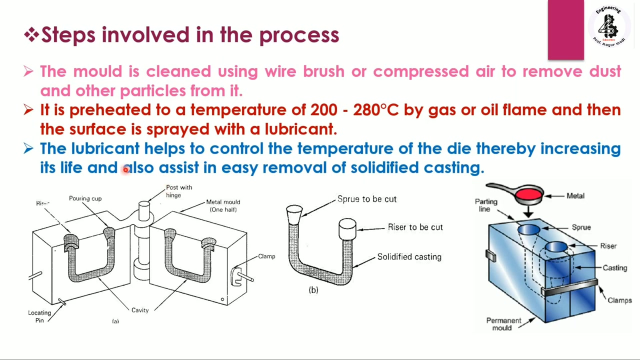 Is cleaned using wire brush, or sometimes it will be using as a compressed air to remove the dust and other particles from it. It is preheated to a temperature around 200 to 280 degree centigrade by gas or sometimes oil flames, and then surface is sprayed with a lubricant. 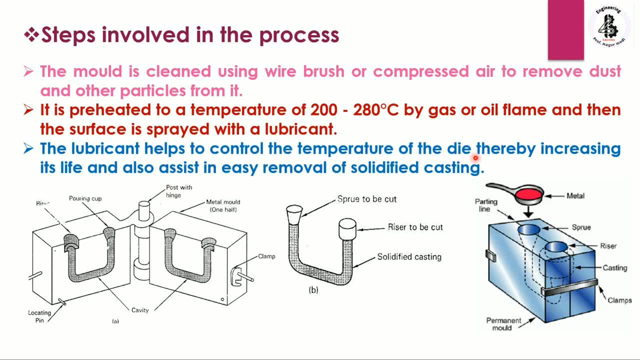 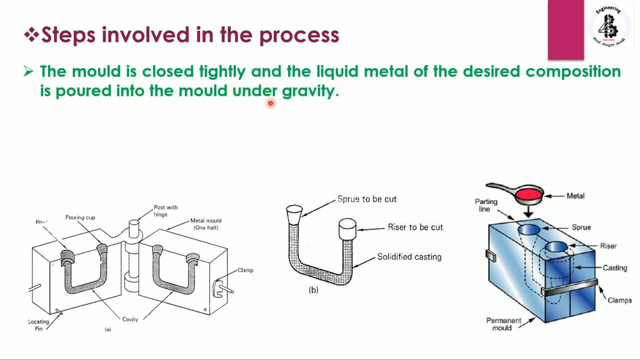 The lubricant helps to control the temperature of the die There by increasing Its life, And also assist in easy removal of the solidified castings. Then, after The mold is closed tightly and the liquid metals of the desired compositions is to be, 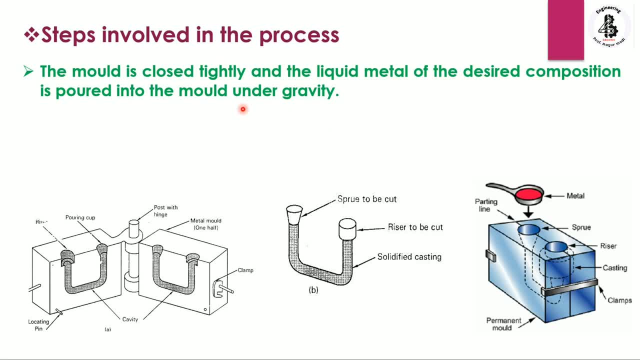 pouring from a sprue towards a cavity with the applications of gravity. After the metal cools and solidified, The mold is opened And the solidified and the casting is being removed. Gatting and the risering systems are separated from the cast part. 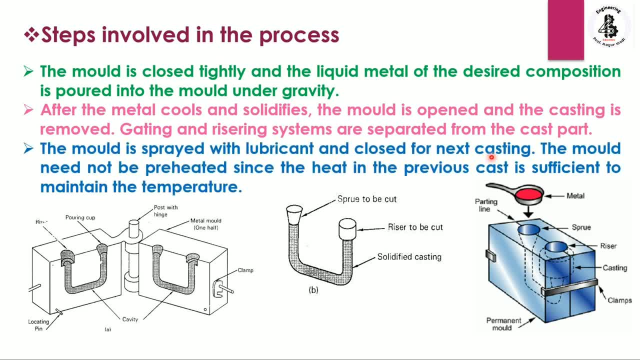 The mould is sprayed with lubricant and closed for the next castings. The mould need not to be preheated, since the heat is previously cast is sufficient to maintaining the temperature. So if there will be the requirements of that preheat, so that will be providing as we discussing. 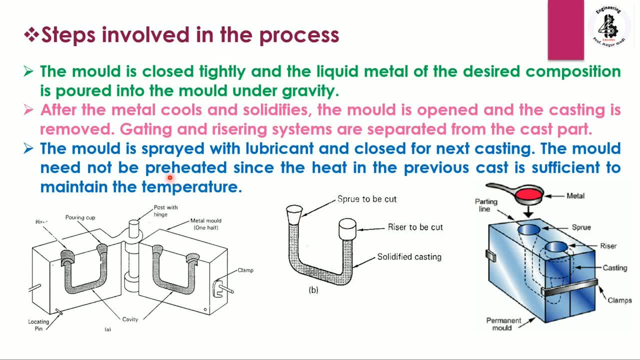 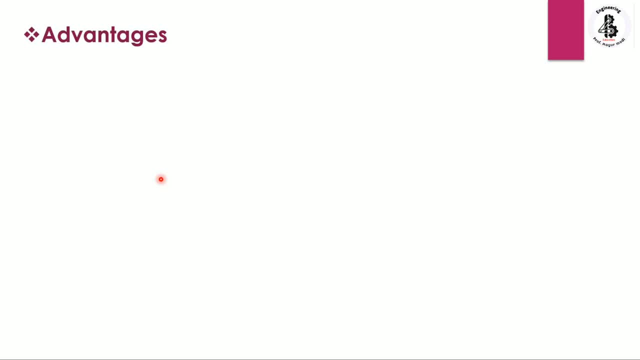 previously. If it will be having some temperatures, there will be the no need to be preheat. Some of the advantages of this process, like good surface finish and close dimensional tolerance, can be achieved, Suitable for mass productions because that will be the permanent mould casting. 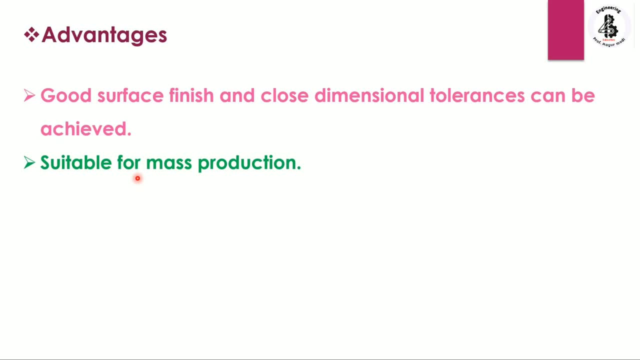 process so that will be only feasible with a mass productions. Occupies less floor space. Thin sections can be easily cast with the help of die casting. Eliminates keel operators. Some of the disadvantages, like initial cost of the manufacturing moulds or you can say die, is high because that will be made with metallic materials.